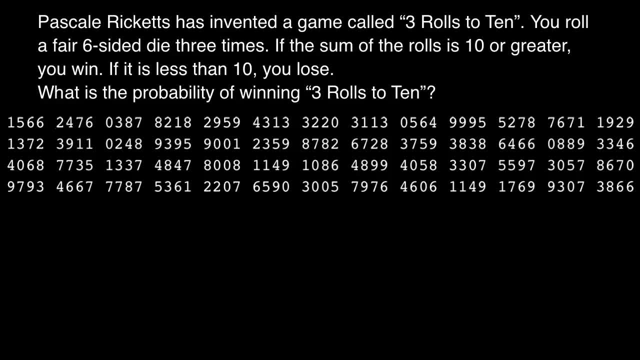 and I'm gonna consider each digit a roll If it gives me an invalid result for a six-sided die. so if it's a zero, an eight, a seven or a nine, I will just ignore that. I will just say, well, that wasn't a valid roll. 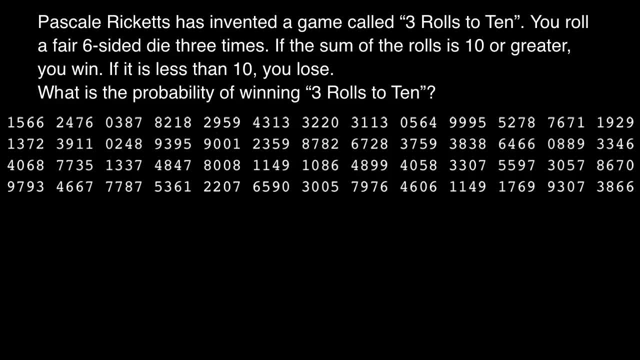 It's like you roll the die and it fell off the table, or something like that. So let's do that, Let's do multiple experiments of taking three rolls, sum them up and we'll see how many we can do to figure out an experimental probability. 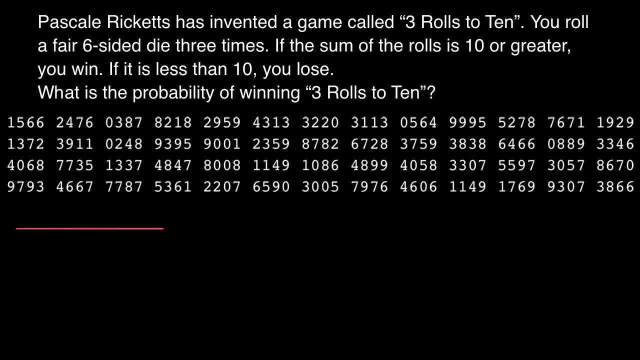 of winning Pascal's game. So let me set up a little table here. So I want space to show the sum. So this is going to be the experiments Experiment. so let me write the sum And over here we're gonna say: did we win? 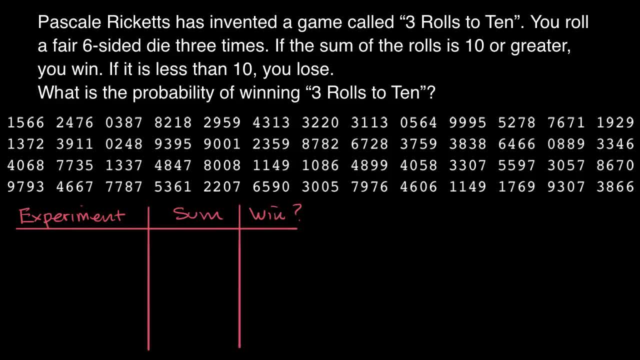 All right, so let's start with experiment one. So our first roll, we got a one. Our second roll, we got a five. We're doing the same thing, We're doing the same thing, We're doing quite well. And then our third roll: we got a six. 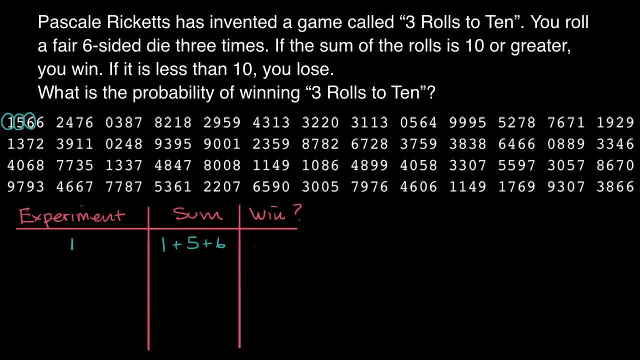 Did we win? Well, one plus five plus six is 12.. Yes, we won. Let's do another experiment. This is going to be experiment two. We can just keep going here. These are random digits, So we have a six in our first roll. 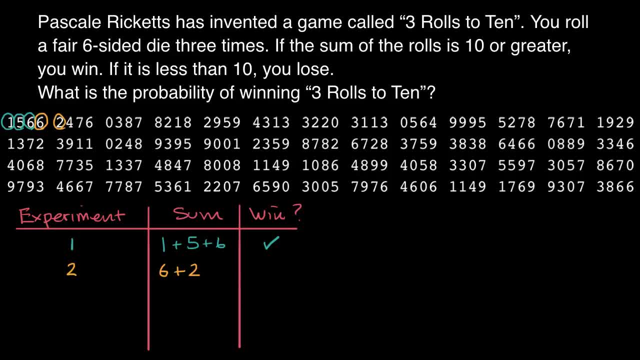 We got a two in our second roll. We got a four in our third roll. Did we win? Yes, once again, this summed up to 12.. So we won. All right, let's do another experiment. So experiment number three. 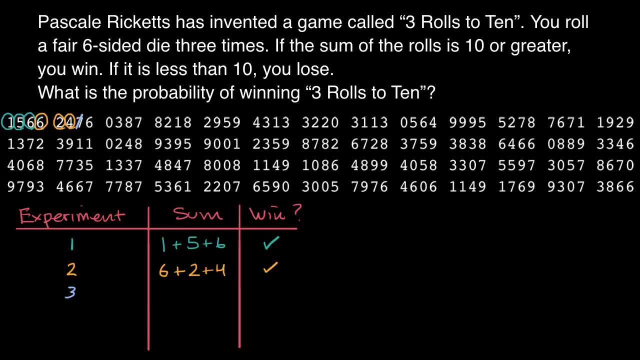 So this first thing is invalid. So this is our first roll. We got a six. And then this is invalid. Our second roll, we get a three. This is invalid, That is invalid, That is invalid. And then in our third roll, we got a two. 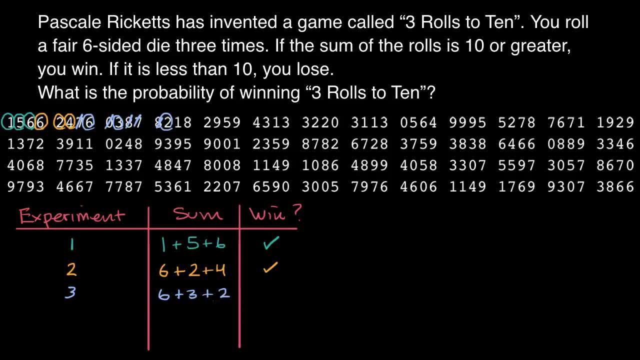 We got a two, So we squeaked by. This adds up to 11.. Yes, that looks like a win. All right, let's do our fourth experiment here. So our first roll: we got a one. This is invalid. 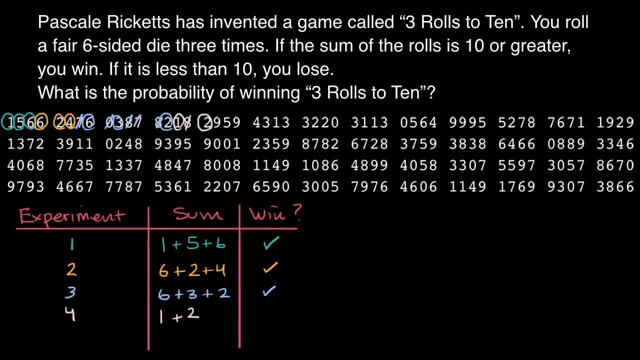 Second roll: we got a two. This is invalid. Third roll: we get a five. Did we win? One plus two plus five is eight. No, We did not win. So that was our first non-win, So let's keep going. 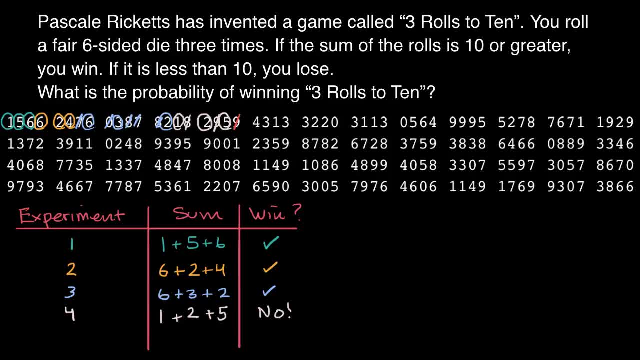 This is interesting. All right, this is invalid. So we're going to have. so this is trial five. We are going to have four plus three plus one. Four plus three plus one adds up to eight. Did we win? No, 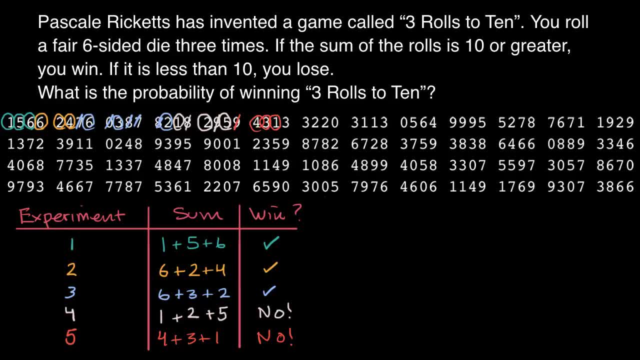 Let's just keep going here. So I'm gonna keep going with my table where I have experiment. I'll do five more trials. So experiment, sum and do we win? Let me make the table. This is just a continuation of the table we had before. 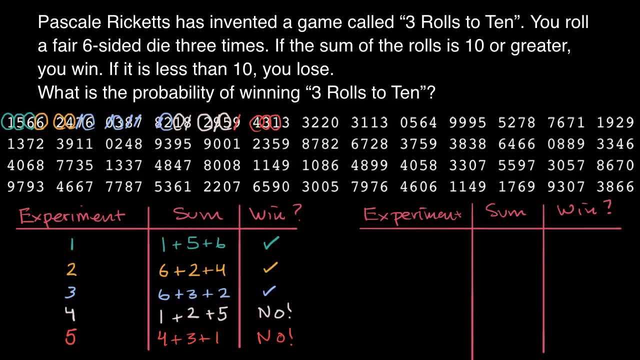 I don't want to go below the page because I want to be able to look at our random numbers here. So we are on to experiment six. Experiment six: we are getting a three in the first roll, a three in the second roll. 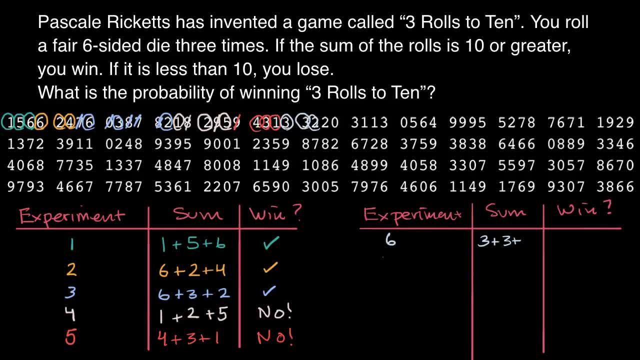 This isn't looking good. And then a two in our third roll. Did we win? No, This is less than 10.. Now we go to experiment seven, experiment seven: We get a two in our first roll. This is invalid. 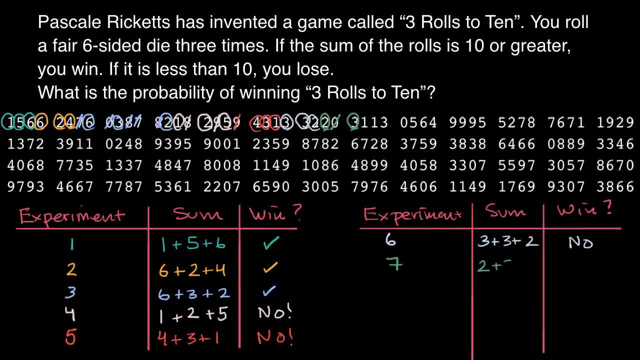 We get a three in our second roll. plus three. And we get a one in our third roll, So plus one. Once again, we did not win. Now we go to experiment. we will go to experiment eight. We get a one in our first roll. 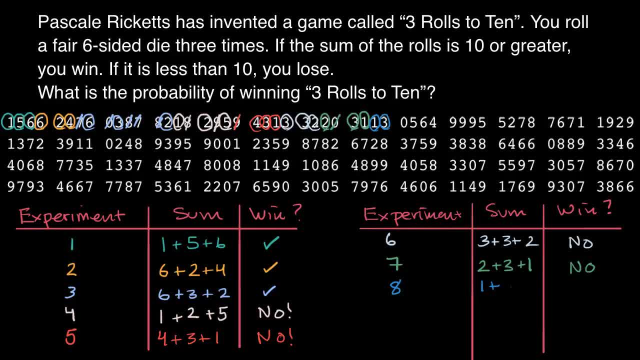 We get a three in our second roll. This is invalid. The die fell off the table. we can think of it that way. And then in our third roll, we get a five plus five. Did we win? No, this adds up to nine. 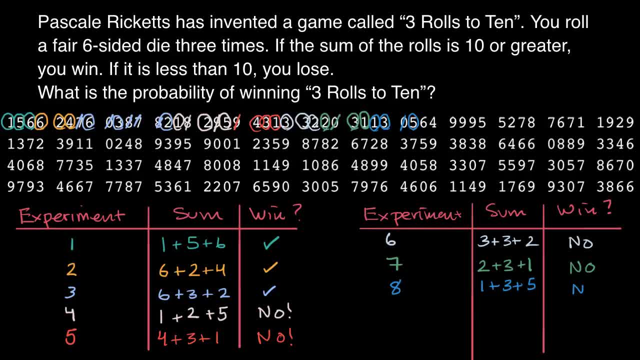 So we had a string of wins to begin with, but now we're getting a string of non-wins. All right, Now let's go to experiment nine. So we get a three in our second roll plus three. Did we win? 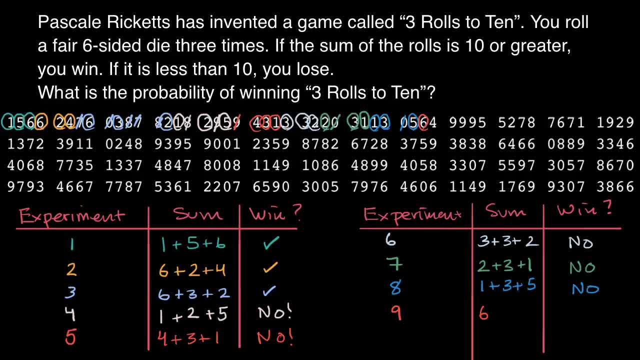 No, We get a six in our first roll, We get a four in our second roll, And then these are all invalid, And then we get a five in our third roll. Did we win here? Yes, we won over here. This is definitely going to be greater than 10.. 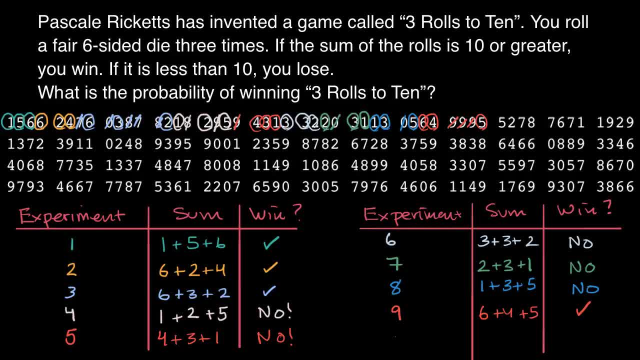 This is 15 here. All right, last experiment, Or at least for this video. last experiment. You could keep going. In fact, I encourage you to after this, to see if you can get a more accurate, a better approximation of the theoretical problem. 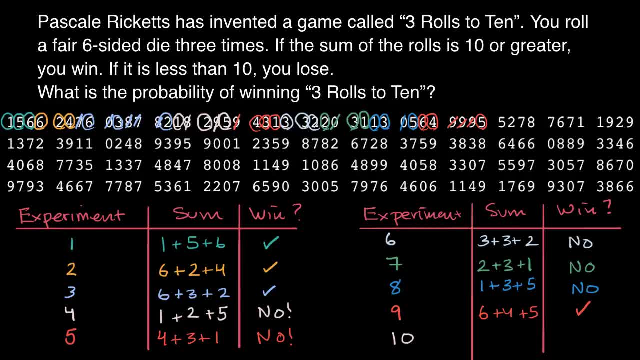 the theoretical probability of winning by doing more experiments to calculate an experimental probability. So here, experiment 10.. First roll: we get a five. Second roll: we get a two. This is invalid, invalid, invalid. Then we get a six. 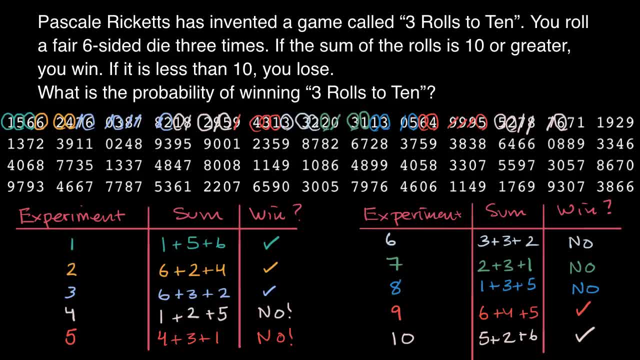 Here we definitely won. So, with 10 trials, based on 10 trials, or 10 experiments, what is our experimental probability of winning this game? Well, out of the 10 experiments, how many did we win? Well, it looks like we won one, two, three, four, five. 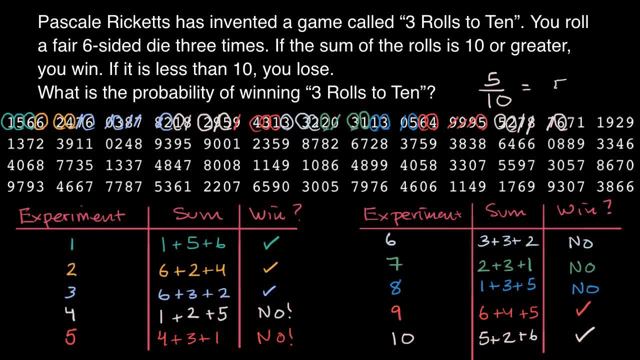 So, based on just these 10 experiments, we got a pretty clean 50%. So do you think the theoretical probability is actually 50%? Maybe you'd want to continue running these experiments over and over. Maybe we'd want to do a computer program. 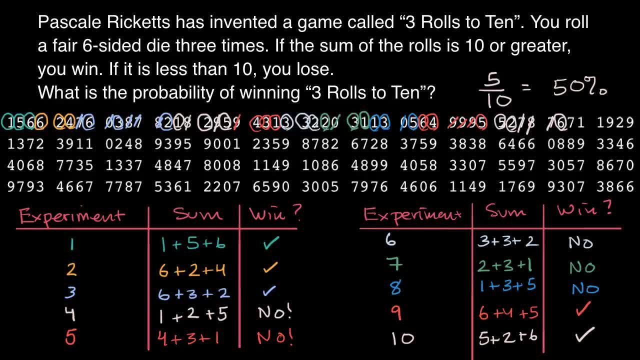 that could run this experiment instead of 10 times, maybe 10,000 times, to see if we can get closer to the true theoretical probability.